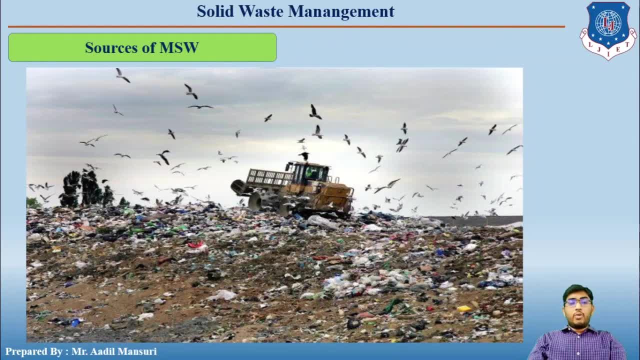 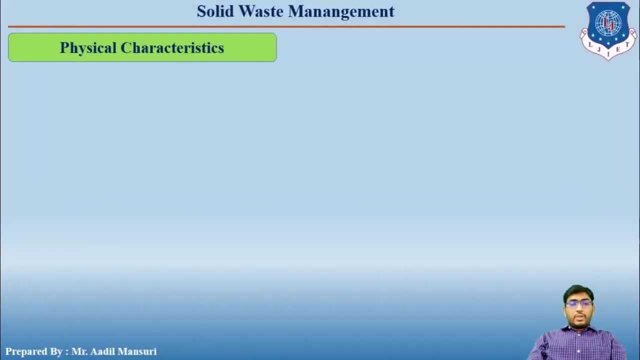 gathered or which are collected, are usually dumped on the landfill sites. Okay, so moving further, let us now start with the physical characteristics of the solid waste. Okay, so there are different physical characteristics. So first one is the determination of the ingredients. right, as we discussed, the different ingredients are plastic. 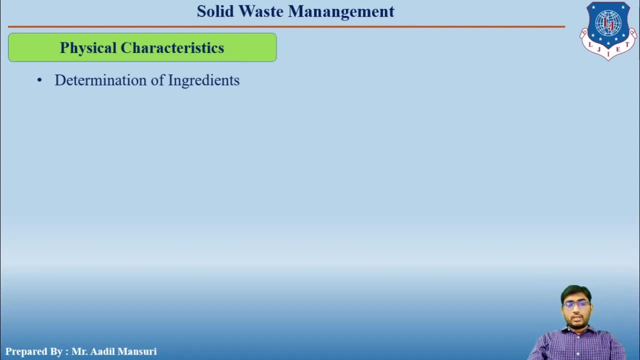 paper, then metals, glass- right, we need to separate those. Then, talking about the bulk density, This is an important point because the knowledge of density is very important for the design of all the elements of solid waste management systems, like storage, transport and disposal. Okay, for example, a known volume of 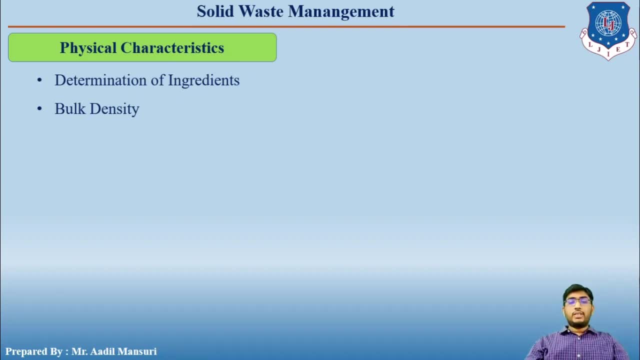 solid waste. for a known volume of solid waste, its density gives us the idea about the requirement of the trucks in the tonnage. Okay, and the density varies significantly from source to the disposal site because of the handling, change in moisture content, densification due to vibration of movements right or disturbance by animal and birds. 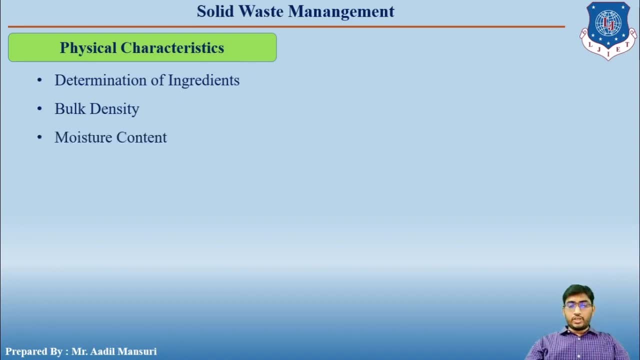 Here. next is the moisture content. So moisture content of the solid waste is expressed as the weight of moisture per unit. weight of wet materials: right, and moisture content varies Generally from 20 to 45 percent depending upon the climatic conditions and level of city, that is, income, group and so on. right and the increase of moisture content. 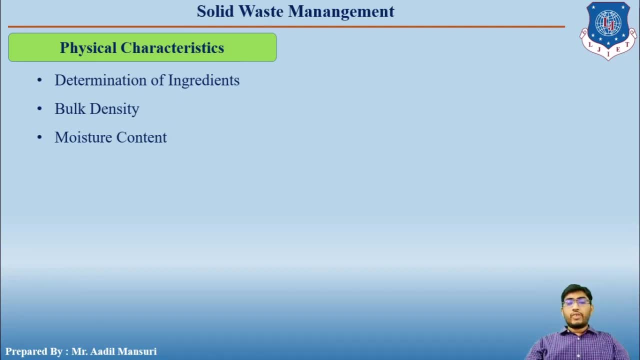 increases the weight and thus the cost of transportation and, as a result, storage section should be taken care of. Okay, then comes the location, from which location you have collected the solid waste. right, then season right, because in monsoon season, because of the rainfall, there will be more formation of leachate as well. clear, then storage time: for how much time the solid 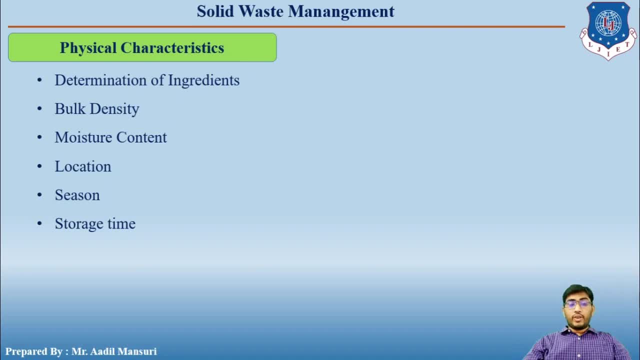 waste has been stored because it will lead to putrefaction because of the anaerobic decomposition or aerobic decomposition right. then there is the equipment that is used to collect the waste, The use right, which are the different equipments used, and processing right, that is, compaction. 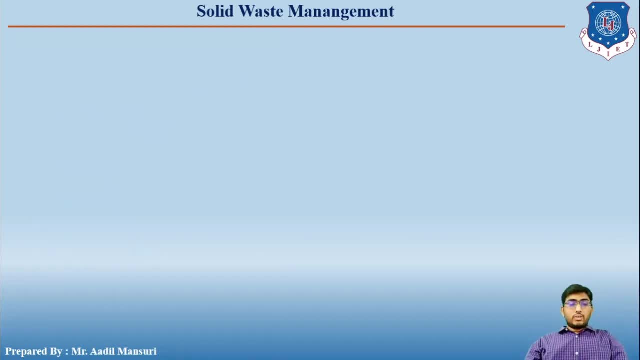 shredding etc. clear. so let us now start with the next topic, that is, chemical characteristics. so chemical characteristics include calorific value. this is of the utmost important right, because the calorific value is the amount of heat generated from combustion of a unit weight of substance, which is expressed as kilocalorie per kilogram. right and the calorific value. 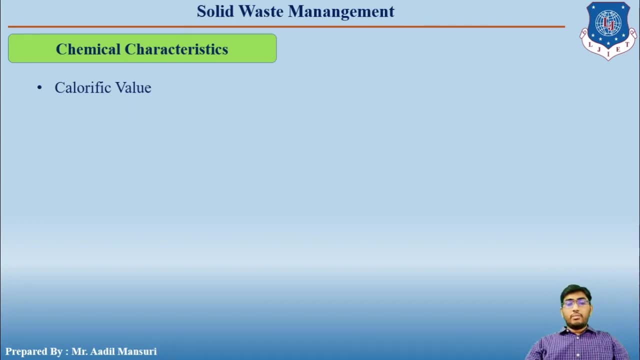 is determined in the laboratory by calorimeter. okay, then the chemical characteristics of solid waste are determined. for assessing the treatment processes, mainly three chemical characteristics are determined, that is, chemical, biochemical and toxicological. okay, that toxological then. chemical quantities of solid waste in indian urban centers are ph nitrogen. 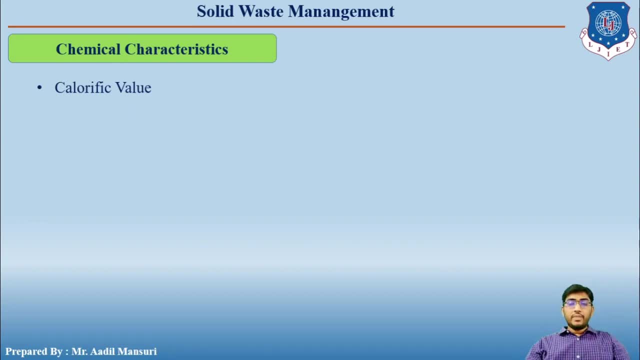 phosphorus and potassium. that is npk and total carbon or carbon nitrogen ratio, calorific value and so on. okay, so these are the different chemical quantities. talking about biochemical characteristics, includes carbohydrates, proteins, natural fibers and biodegradable matters. and last, talking about the toxic characteristics, include heavy metals, pesticides and insecticides. 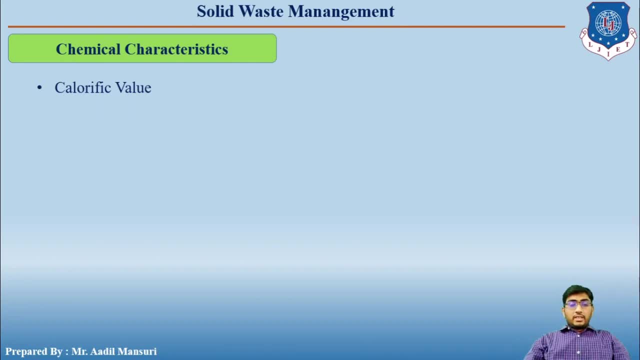 right now. consideration of lipids, that is, fats, oils and greases, should also be taken, as they are of very high calorific value, about 30 thousand kilo calorie per kg right. these days, synthetic organic materials like plastic have become a significant component of solid waste, which is 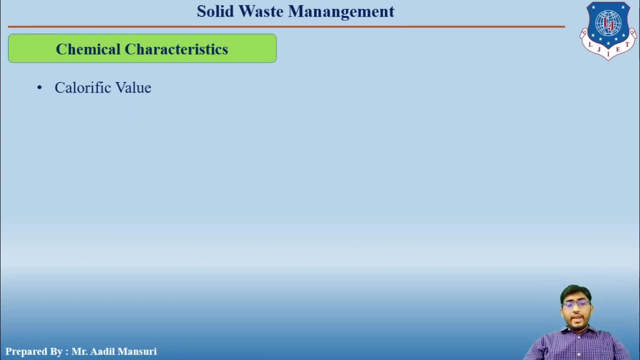 accounting for five to seven percent in India. the plastic is non biodegradable and thus poses a great problem. right. it chokes the drains and if it burns it produces poisonous gases. like the thin plastic sheet and bags are not recycled, as the cost of making it dirt and oil free makes the process uneconomical. right. 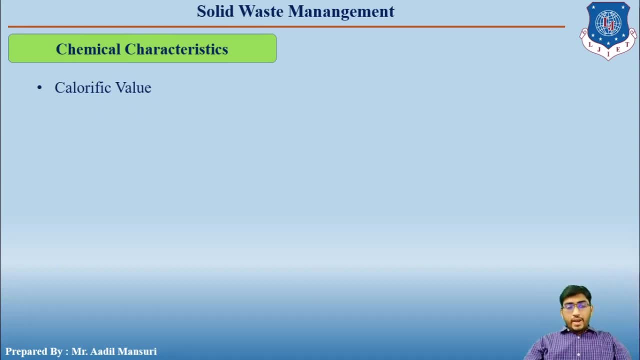 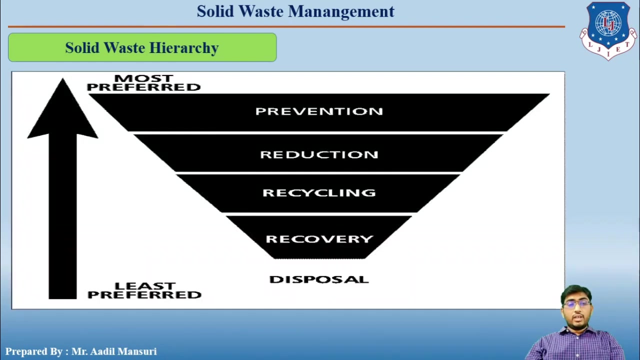 so all this consideration of characteristics are required to design, conceive and assess the most appropriate ways of transportation and the requirements of treatment, extraction of energy, the safe, sanitary way of disposal for the protection of the environment. yeah, so let us now talk about the solid waste hierarchy. so, my dear students, this is the. 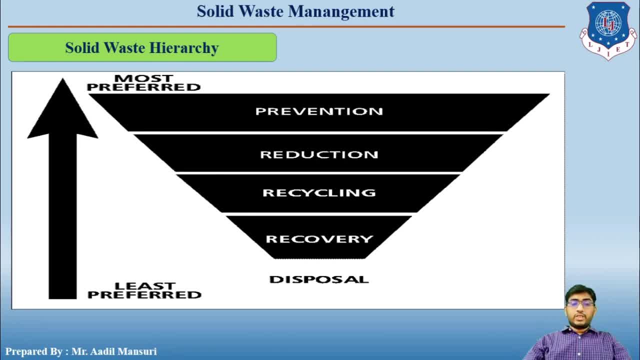 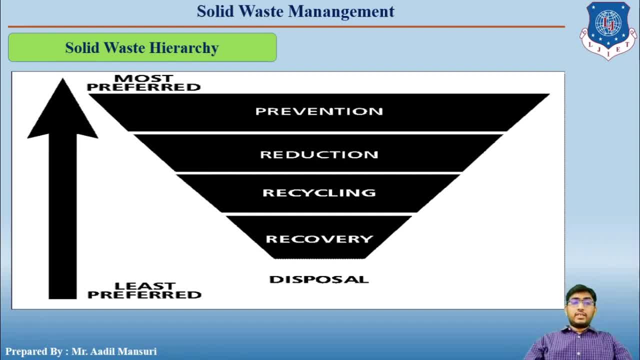 such material right now. if it is compulsory to use those materials, then try to reduce the use of those material. okay, that is the reduction. fine, if it is not possible, then try to recycle the used material. okay, and then if recycle is not possible, then you can go for recovery. and finally, if 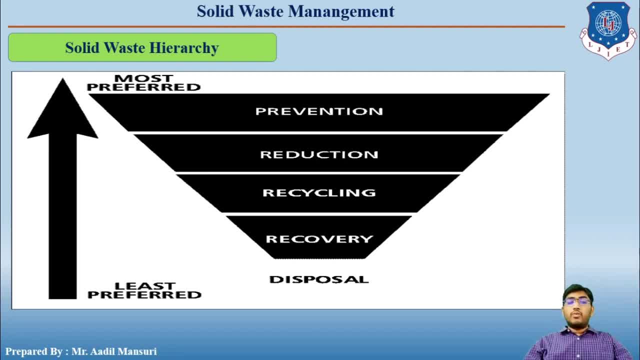 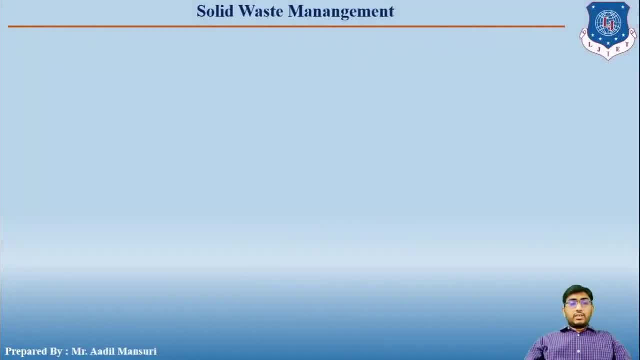 nothing is possible, then you can go for disposal of the solid waste. okay, so next talking about the components of solid waste management. so first one is the Collection of Roberts waste, identification of waste and its minimization at the source, directors, end storage at the size of site of collection, transportation. 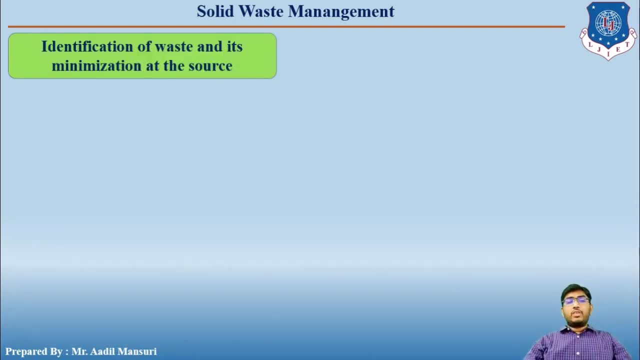 bulletin and an entity and disposal. okay, so let us talk about identification of waste and its minimization at source. okay, so the minimization of the waste production is the various routes. the graceful waste management seems easy to follow. to be so in an individual, the best strategy, correct. and for this, first of all, the process should be such that there is 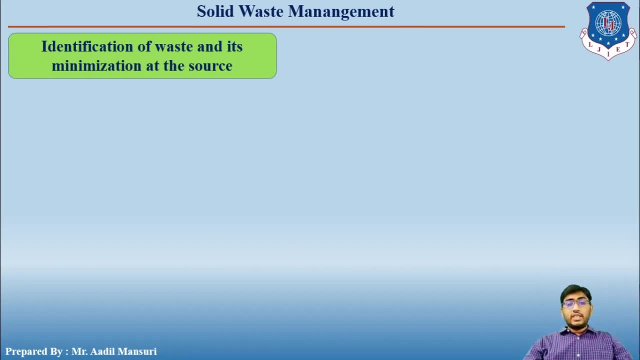 at least production. there is a least production of the waste. okay, then the next step is to reuse the remaining waste in the same process. this reduces the cost of transportation. okay, then, these methods can be adopted on a large scale as well, but for that the waste is first collected. 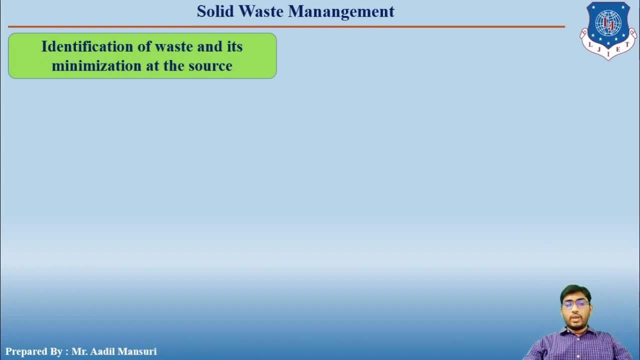 transported and then utilized. okay, this incurs a large cost, so it is always preferable that, if the waste production is minimized, the or the waste is reused or recycled at the source itself. thus the 通 tio planning, changing attitude. sometimes special investments are also needed, and most 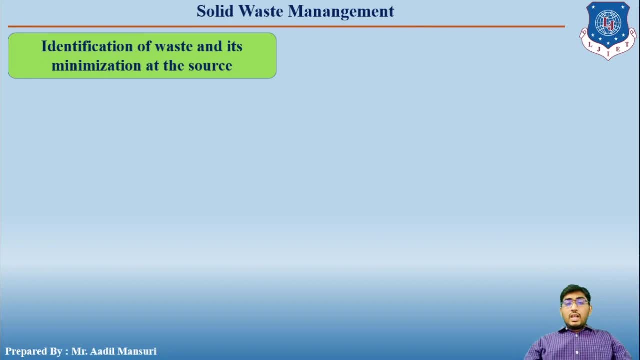 important is the commitment right. the self-motivated will reduction of waste generally not possible. okay, the self-motivated willing reduction of waste is generally not possible. so strict enforcement of law should be there right and the reduction and the reuse, recycle should be given incentives from government in the form of tax. 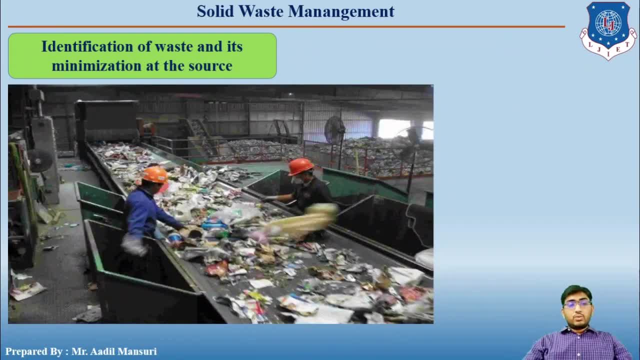 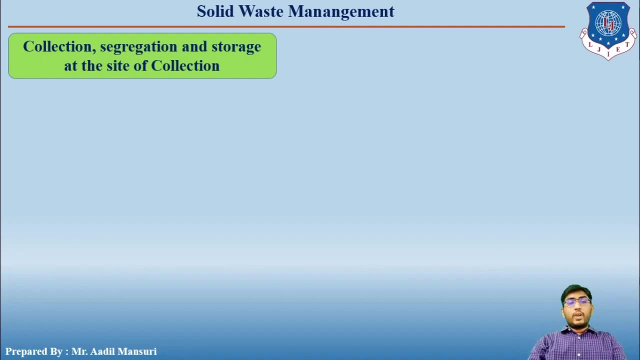 reduction or loans. okay, so this is what, uh- identification of waste and usually segregation- is done. okay. then next is collection, segregation and storage at the site of collection. so the main problem of solid waste management is the collection of solid waste. the household waste consists of all type of general waste right, and at present there is no scientific, clean, hygienic. 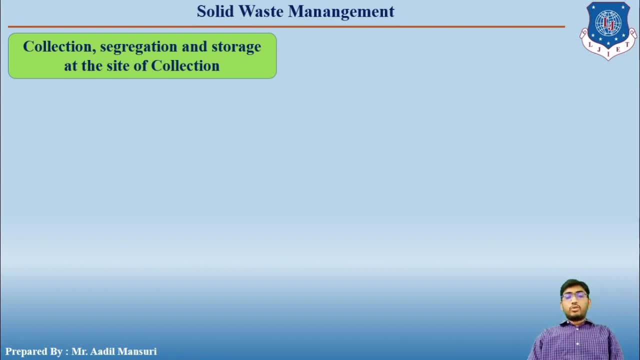 efficient practice of waste collection. in most of the cities of india, including the metro cities, right now, the industrial waste is also handled in the same way, and the collection and storage of the waste is most neglected operation in any industry, right? so the best way would have been the segregation of waste at the 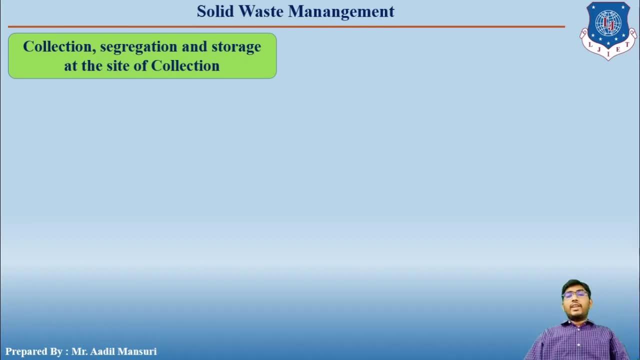 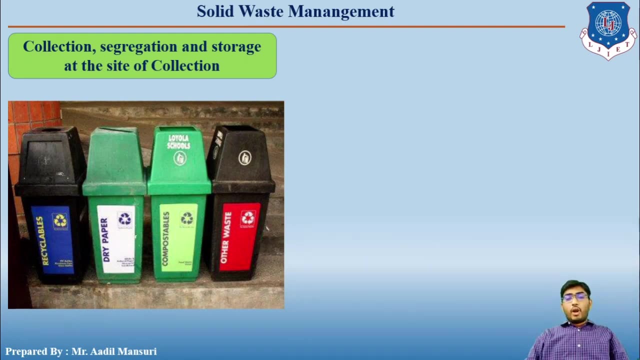 generation point. segregation means collecting it in different beans or plastic bags. you can see the picture right and the domestic waste can be broadly separated as reusable- that is, plastic, paper or metal- and non-reusable- right, and the non-reusable may have organic matters like kitchen waste or 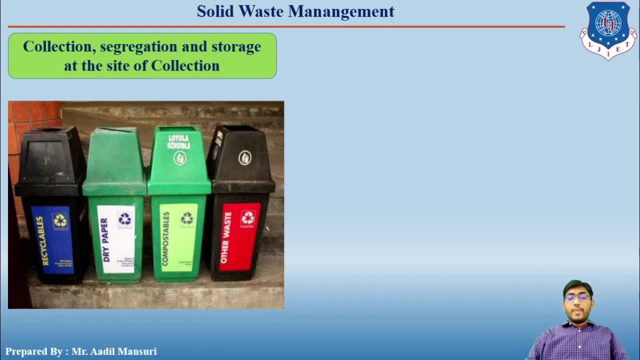 inorganic matter, like dry food, like killing cars, like dust or dirt, right, and the organic matter is liable to decomposition and those requires immediate attention. right then, this separated waste should be regularly collected by the worker directly from houses at some well-defined point of time. right then, it should be transported in covered vehicle. 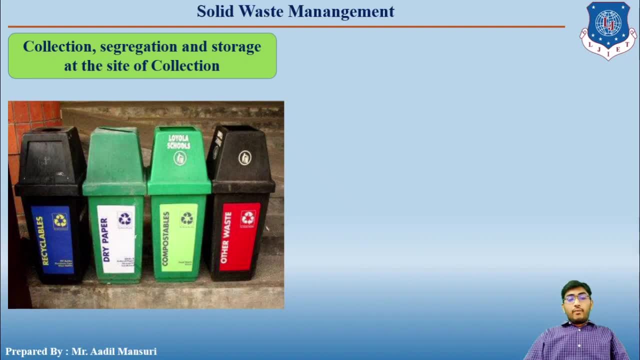 to some waste collection depot, depots for utilization, transportation to different sites. the organic waste can be used for the production of biogas. biogas or for the extraction of the energy incineration right that is controlled burning, or making organic compost or vermicomposting right. so this 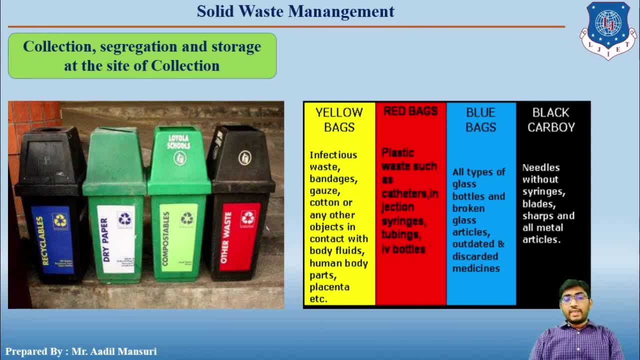 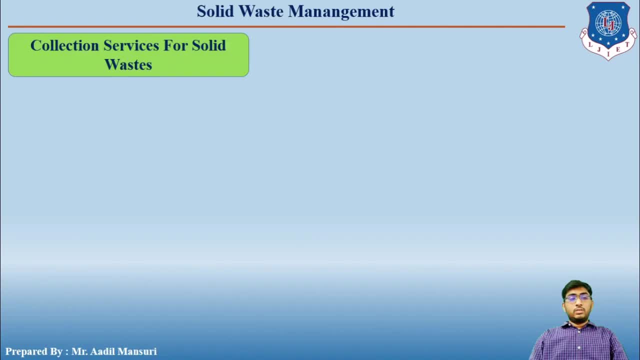 is a color coding- yellow bags, red bags, blue bags and black bags- clear. so let us talk about collection service for solid waste. so first one is the curb service, right? so, although a variety of collection services are available, the most common are curb, alley and backyard collection. 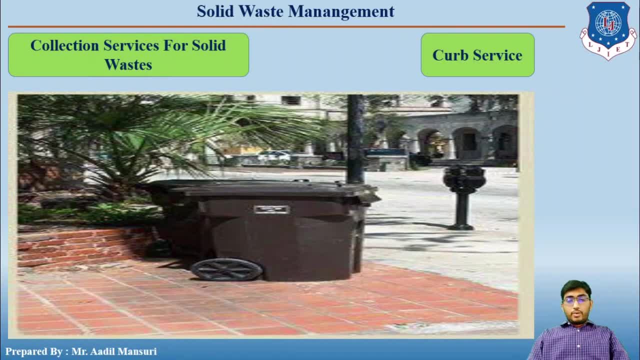 so let us talk about the collection service for solid waste. so this is the curb service, right? so curb collection has gained popularity because labor cost for collection can be minimized and in the future it appears that the use of large container which can be emptied mechanically with an